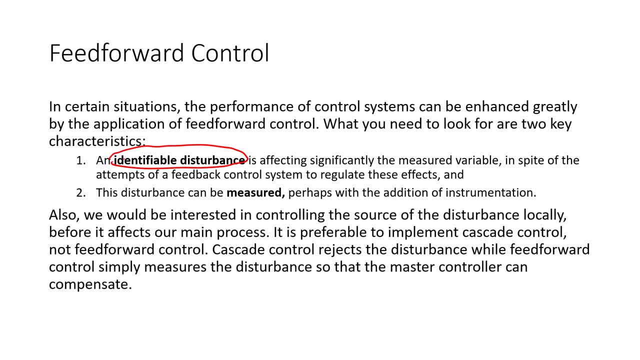 Okay, so we also want to be able to control the source of the disturbance, locally, before it affects the main process. We might consider a cascade controller instead if we have the same final control element that is able to control that disturbance and the process. Okay, so cascade control is preferable if we have the right scenario, but we can use feed forward controller if it isn't. 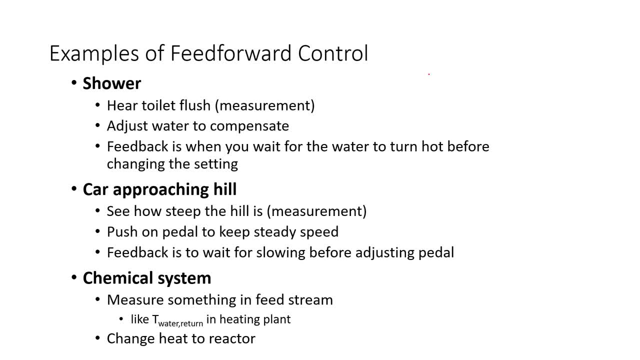 Okay. so examples of feed forward control. We might have, for example, a shower. Okay, we're taking a shower and all of a sudden we hear the toilet flush and we know that the cold water pressure is going to go down and so it's going to be hot, and so we might jump out of the way. 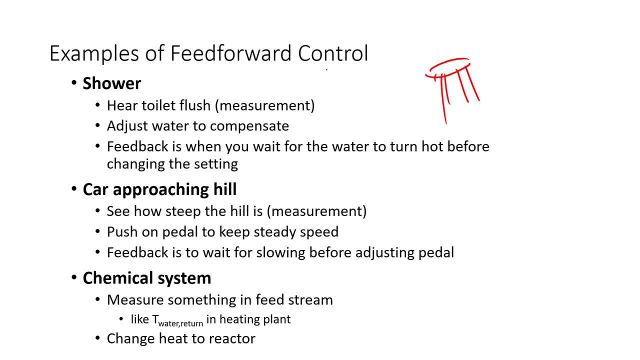 Okay, so that's an example of when we would apply feed forward control. We hear a disturbance happening and we understand that something's going to change in our temperature. Okay, also, a car approaching a hill. Okay, so I have an automobile and it's approaching a hill. You know, someone that's driving the car might anticipate this hill and adjust the gas pedal down to compensate, to know that I need to have more fuel going into my engine in order to maintain a speed going up this hill. 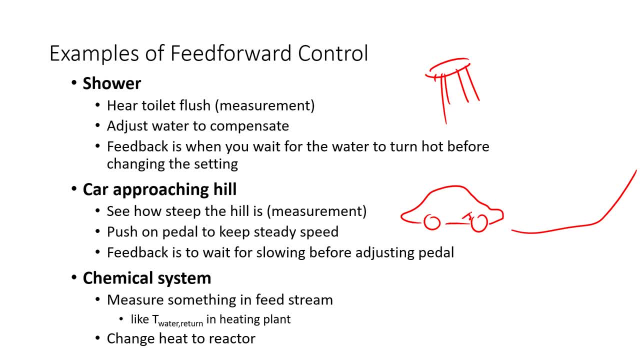 Now feedback would be: if you didn't know this hill was coming and all of a sudden your car started slowing down And you would apply more gas to compensate for the slowdown, With a feed forward, you can anticipate that disturbance and potentially not have that air in the speed and have an improvement in terms of disturbance rejection. 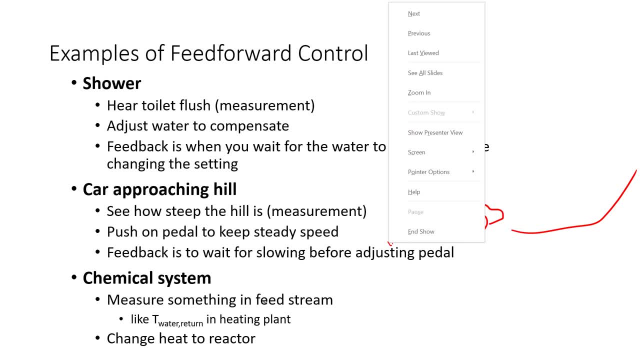 Okay, chemical system. We want to measure something, maybe in a feed stream, and then change the heat to the reactor, for example. You'll compensate for this disturbance before It starts driving me- my process conditions away from the desired set point. 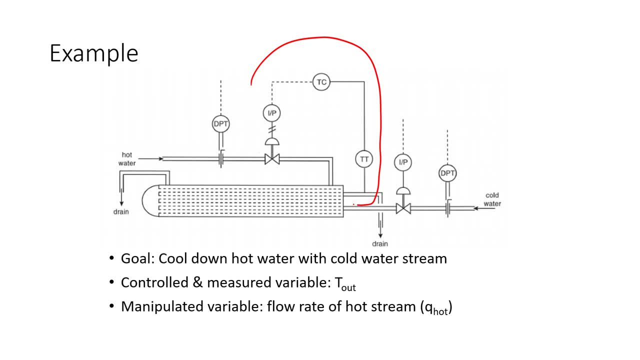 Okay, here's an example. This is a standard feedback control system here, where we have a, you know, hot water is coming in and then it goes through this heat exchanger. Okay, this is on the shell side and then on the tube side we have the cold water. 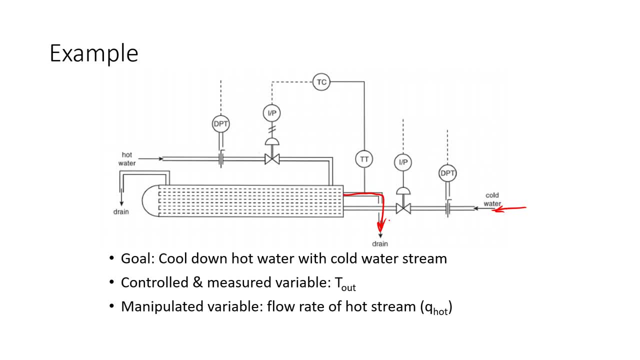 Okay, cold water coming in And then leaving right there. Okay, so the goal is to cool down hot water. Okay, so we want to try to cool this down before discharging it And we're going to use some cold water, maybe coming from a, you know, cold water supply, to do that. 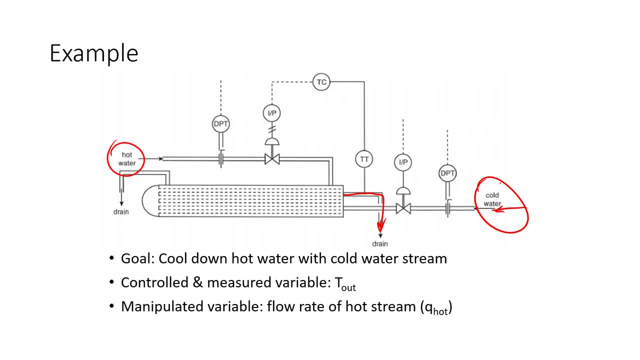 Okay, now we, for whatever reason, we don't want to just add the cold water to the hot water. We want to keep those two separate. Okay, so we have a controlled and measured variable, which is our temperature output. Okay, so it's going to be this: the temperature of this cold water coming out might be our one that we're trying to measure. 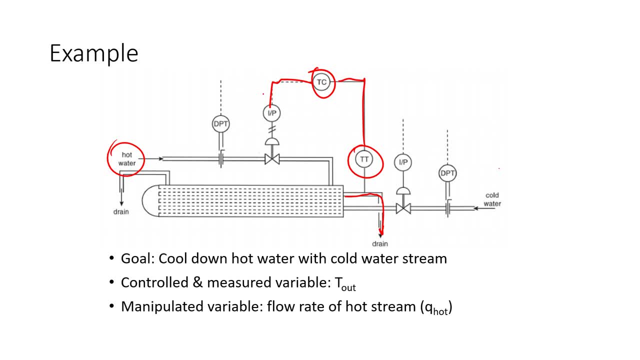 And then we have a controller that's going to adjust the hot water coming in. Okay, so the manipulated variable is the flow rate of the hot stream. Okay, this hot stream right here. Okay, so that's our. Okay, so that's our. 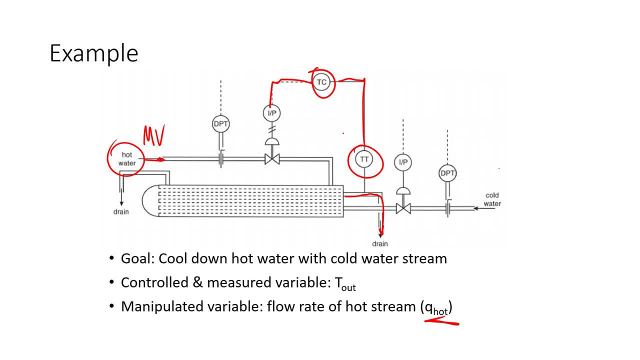 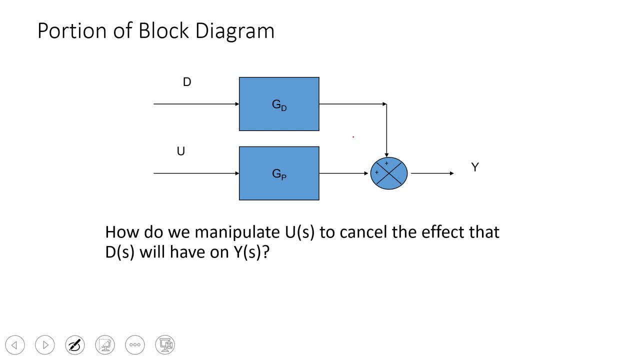 Okay, there's our feedback control loop. Okay, so we have a disturbance. You know we might have a changing cold flow rate. Okay, so that would be our disturbance And our manipulated- this is our manipulated- variable: the flow rate of the hot water. 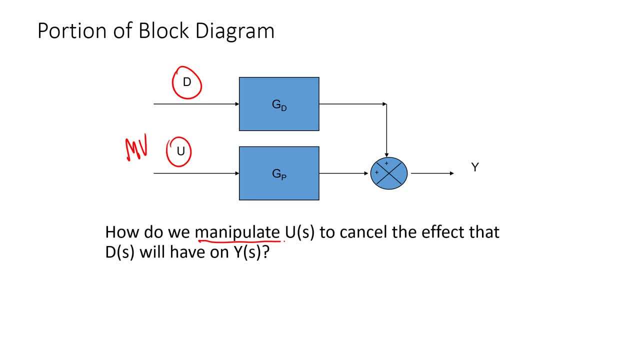 Okay, so we, how do we manipulate? Okay so we, how do we manipulate You to cancel the effect of our disturbance? So we're going to measure this, We're going to measure the disturbance and we want to have our Y equal to zero. 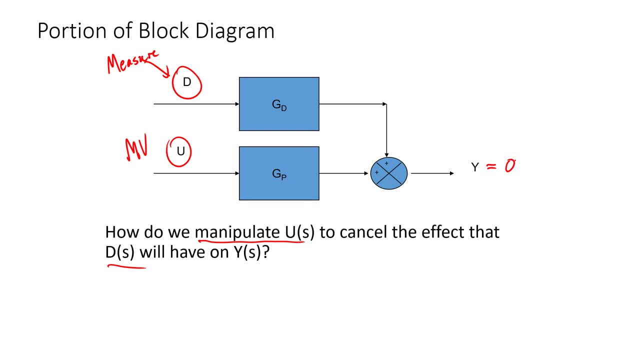 We're going to be a setpoint. We don't want that to change from, maybe, a zero setpoint. Okay, So, in terms of deviation variables, Uh, we're going to say that that equals zero. okay, so we want to have a feed forward controller. that we're going to. 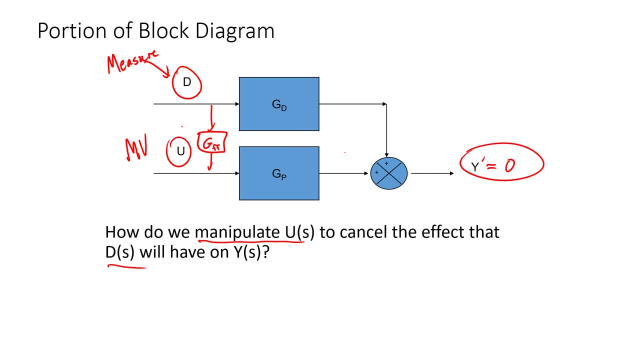 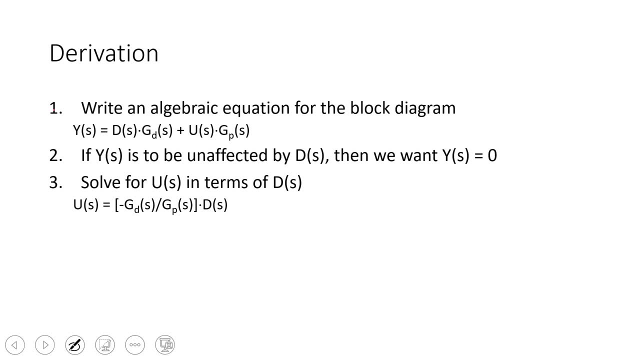 add right here, and the question is: how do we design that feed forward controller so that we get a perfect control? okay, so first of all, we want to write an algebraic equation for the block diagram. these two are going to be in parallel, so I can just add those two together and if Y is to be unaffected by the disturbance, 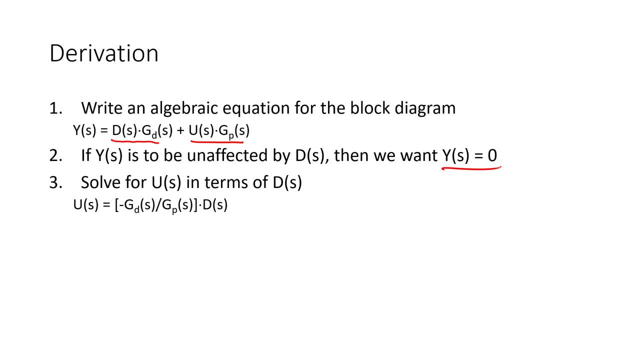 then we want this, this Y, this output to be equal to zero, and then we just rearrange and solve for U. okay, so I'm going to take this right here and just solve for U, and that's what I want my U value to be, and that's that is going to. 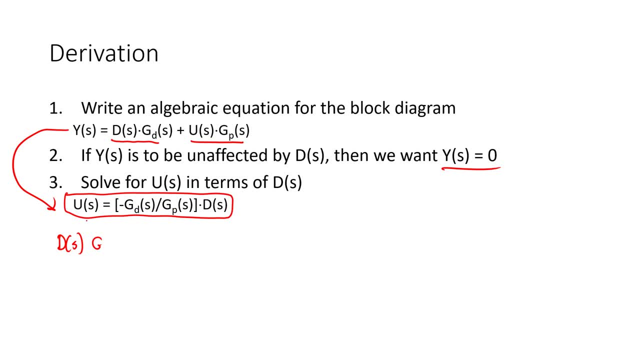 be my disturbance times, my feed forward. okay, so that's going to be my U, my input signal, only to be my disturbance times, my feed forward controller. so this is how I design a feed forward controller. so the disturbance is going to cancel out, and so my feed forward controller is going to be my disturbance transfer function. 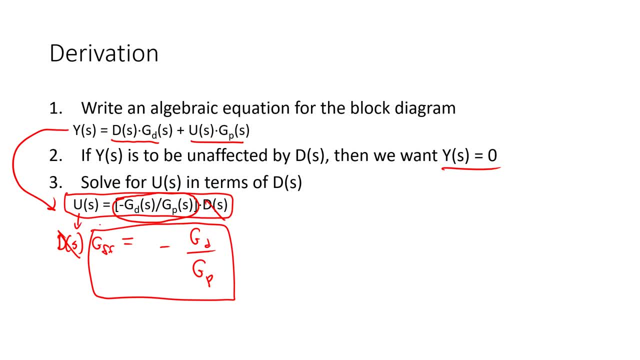 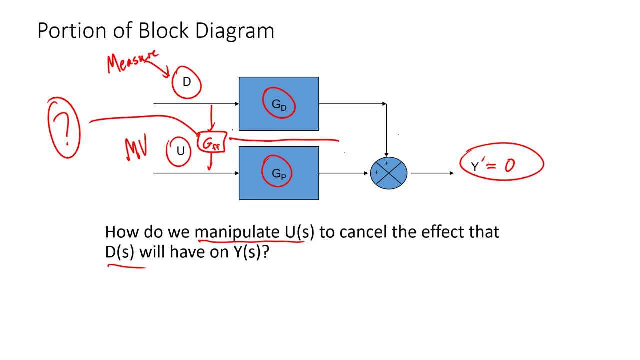 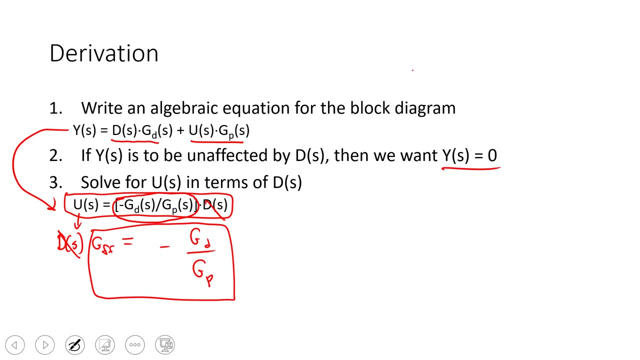 divided by my process transfer function. so let me just go back here. here's my disturbance transfer function and I'm going to divide it by my process transfer function and take the negative and that's going to be equal to my feed forward controller. okay, so let's just look at. 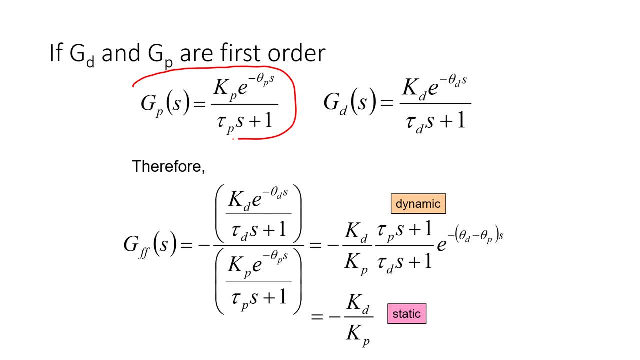 this now we have. you know, just this is a first order plus dead time model of my process and my disturbance. and so if I just take the ratio of these two and combine them, okay, so this one's going to come up into the numerator, so that's. 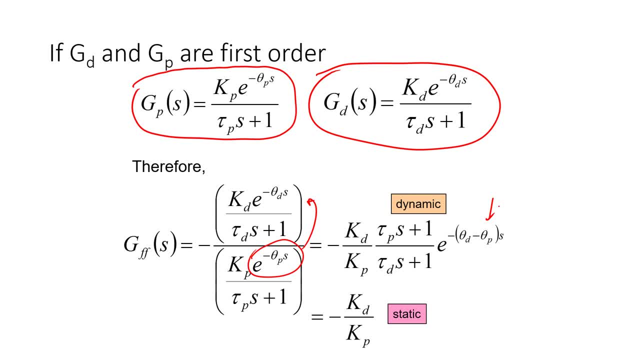 going to give us a positive sign here for my theta P, or if I put in this form that I have: have it like this, okay. and then I have this one that comes up to the numerator, okay, right up here, and that's still in my denominator, and then 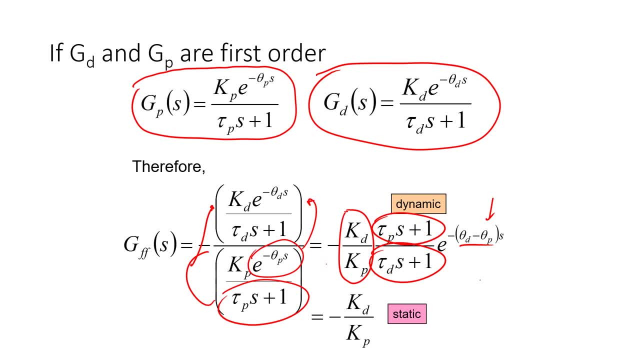 I have a ratio of these gains as well. now, a lot of times we don't implement a dynamic feed forward controller. we'll just, since we're going to have a dynamic feed forward controller, we'll just assume that those are approximately equal to the tau P, beta p and tau d. 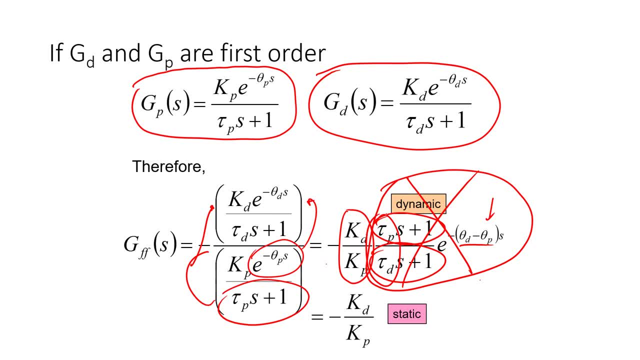 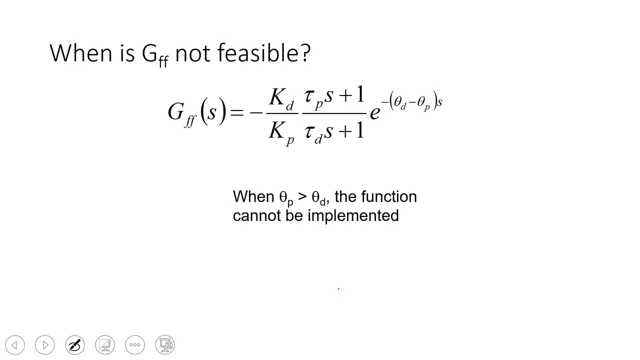 are approximately equal. okay, those are very similar. and if these are also fairly similar, then we can get away with a static feed forward controller, which is much easier to implement. okay, so when is dynamic feed forward control are not feasible? okay, it's when you know. theta P. 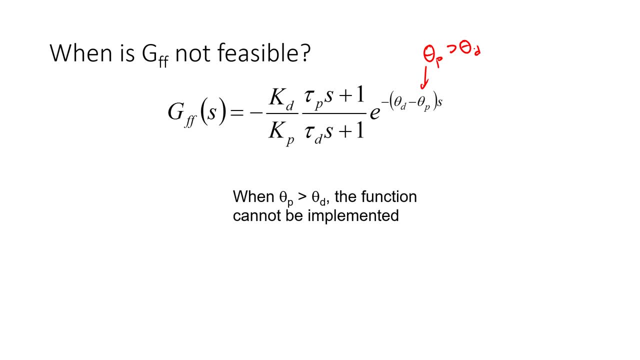 okay, so when is dynamic feed forward control are not feasible? okay, it's when you know theta P and going to be greater than theta D. my dead time for my process is greater than my dead time for my disturbance, and what that means is that we'd want a controller. 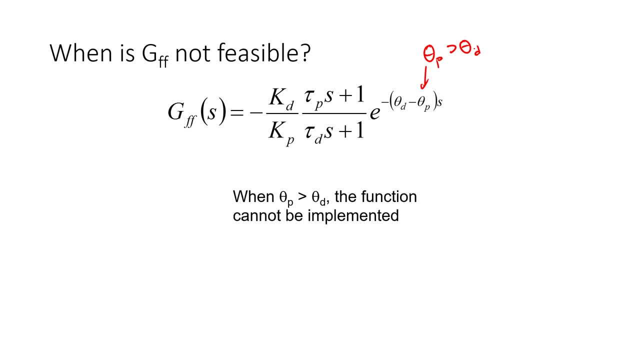 that would be able to act, you know, in anticipation of a disturbance before it's even measured in the, you know back in the in the future time. so it's not physically realizable. we can't necessarily anticipated disturbance before it's going to happen. if you can, this might be possible to implement. but 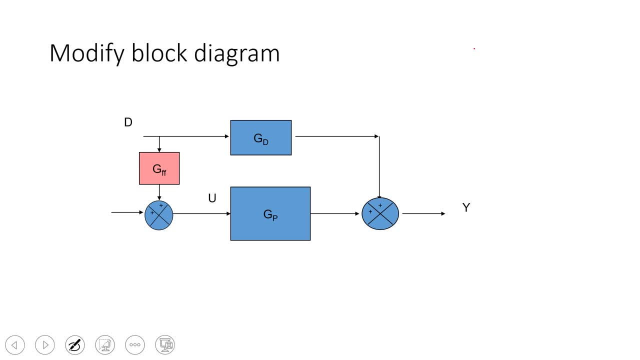 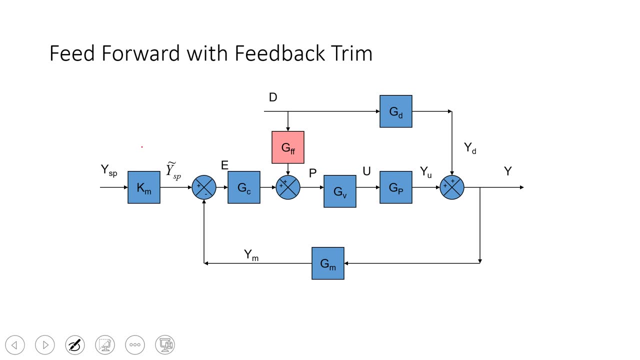 most times you can't okay. so here's our modified block diagram with our feed forward controller right here, and this is with feedback trim. so this is the big picture and where the feedback, the feed forward controller, fits into this. so we're measuring our disturbance and then we're going to 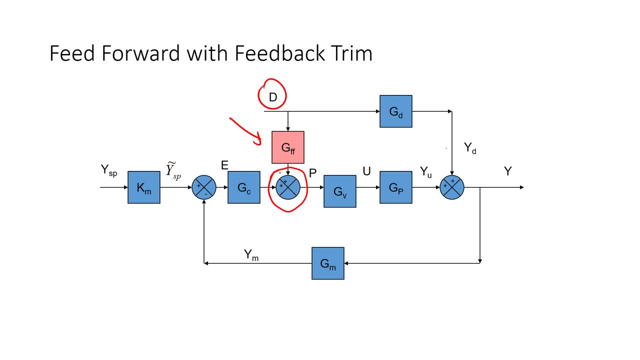 change the feedback trim. so we're going to change the feedback trim. so we're going to change the feedback trim. so we're going to change the controller output proactively, based on that disturbance, to reject it. okay, to compensate for the disturbance and how it's going to eventually affect our process, we're. 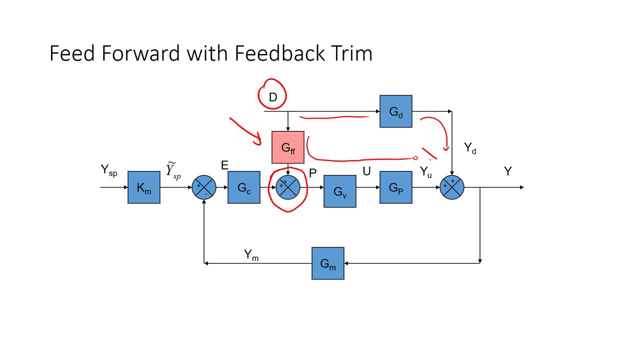 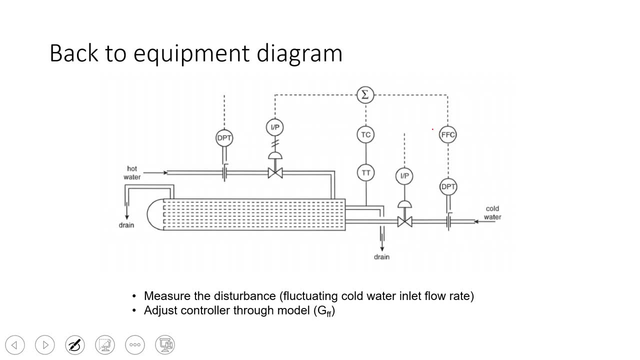 going to send kind of a counteracting signal here to counteract that disturbance, and so we stay on the set point. okay, so let's go back to this equipment diagram. we're going to implement a feed forward controller now, this one. I'm just going to say that this is a flow. 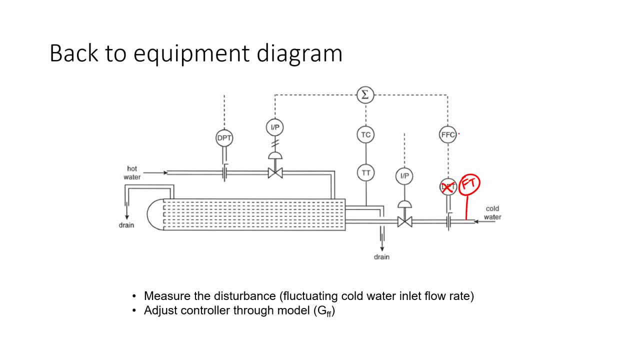 okay, so I'm going to measure the cold water flow coming in. that's going to be my disturbance, and a lot of times we say that that's just going to feed directly into my temperature controller. I'm just going to add something to my PID controller that is going to be a feed forward. okay, or you can write it this: 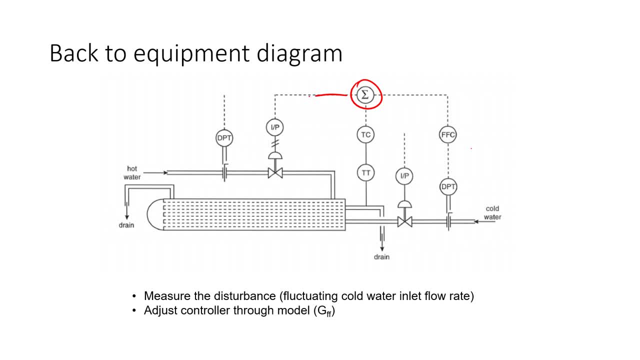 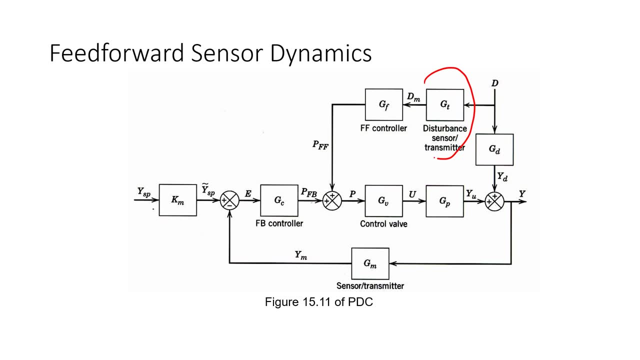 way instead. instead, as they just add up and that gets sent to the valve. okay, so here's feed forward with sensor dynamics, just so. the one change here is that sometimes you have some dynamics of your sensor. you might need to include a transfer function there. okay, so let's do the disturbance rejection performance. 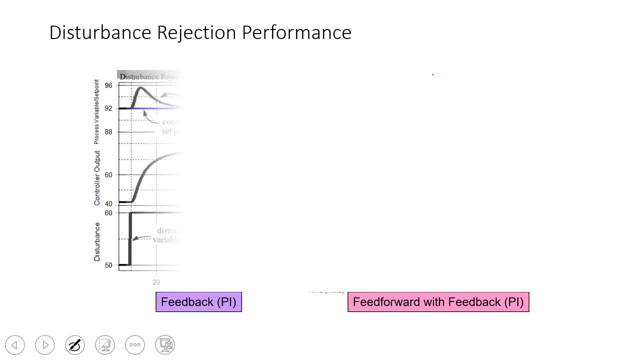 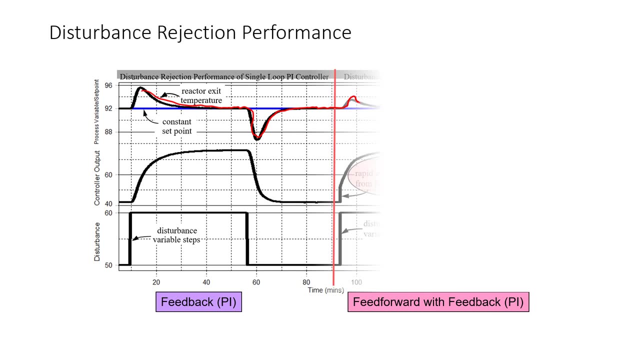 here's an example: okay, and you can see that this is going to start tracking. there's a disturbance. you know these are large without the feed forward and then with the feed forward it's going to be smaller because it anticipates- okay, it anticipates and the controller acts a little bit. an anticipation of 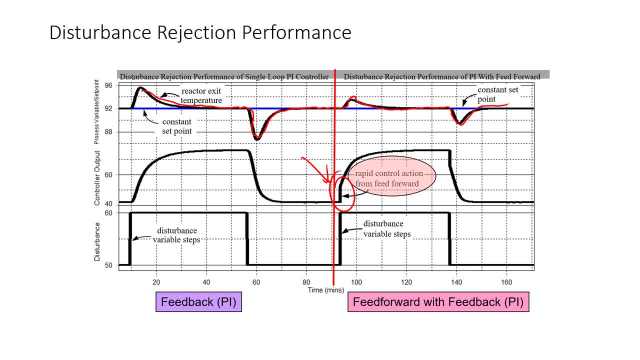 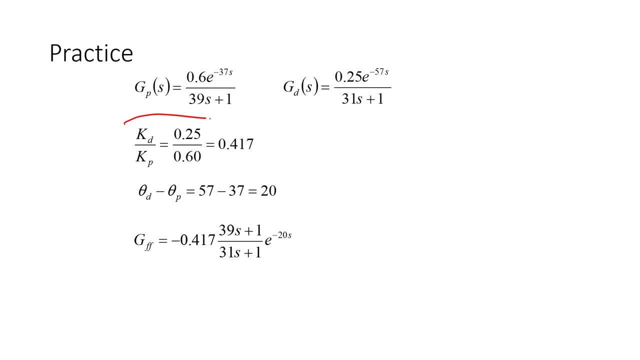 that disturbance, and so it doesn't drive it away from the set point as quickly. okay, here's a practice problem here, just with some numbers. okay, I come up with my static feed forward, which would be the negative of this. okay, negative, negative, and that would be K feed forward. or if I had my 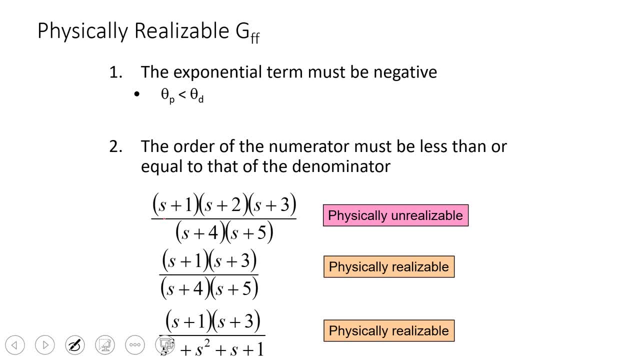 dynamic feed forward. there is the answer. okay. so it's another case where it's going to be physically unrealizable if you have a higher order polynomial in the numerator than the denominator for our feed forward controller. so you got to watch out for that. sometimes you can make it just a first order plus dead. 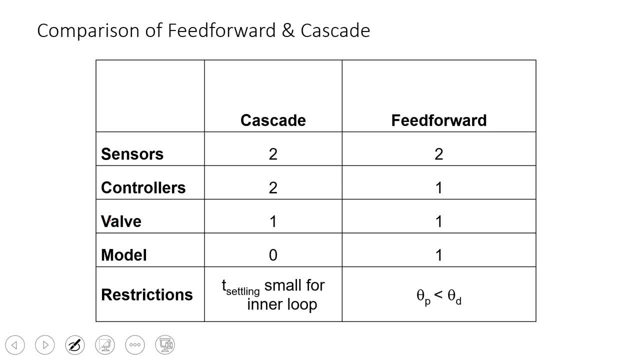 time approximation to that. okay, just a summary of feed forward and cascade. cascade is a general instruction limit, okay. okay, that gives the controller there's a 素, and then use feed and read forward. the evaluation for whom, where they were righting time, often contained one valve, zero models. okay, we're rear model. you don't need a model there, disturbance model, for example- and you have to have one sensor- seriespar haller, very similar. the one difference is that you only have one controller, that you have a disturbance model as well. you have that restriction on the dead type that I mentioned earlier. okay, so recommendation: use cascade when you can. then give us an opportunity here. if i can, can give you a 60- minute. 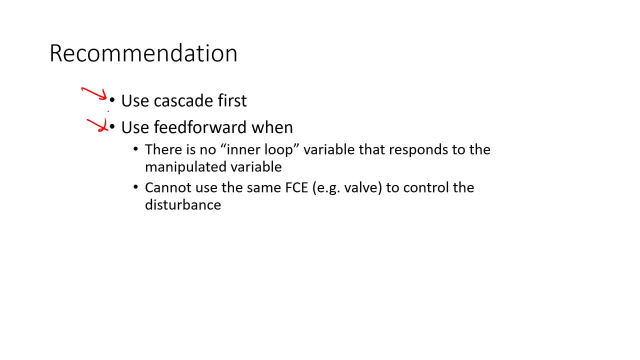 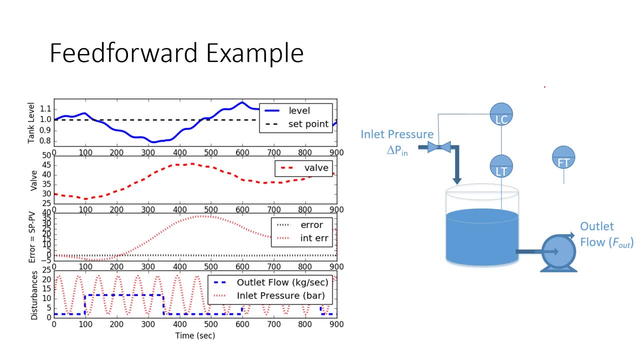 when there's no inner loop and you cannot use the same final control element, for example valve, to control the disturbance. here's a feed forward example that I'll cover next and do a little bit of a problem here with this tank. so just look on the course website for this example. I'll go to that really.